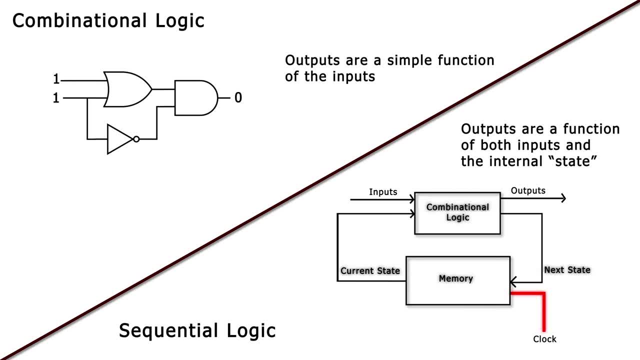 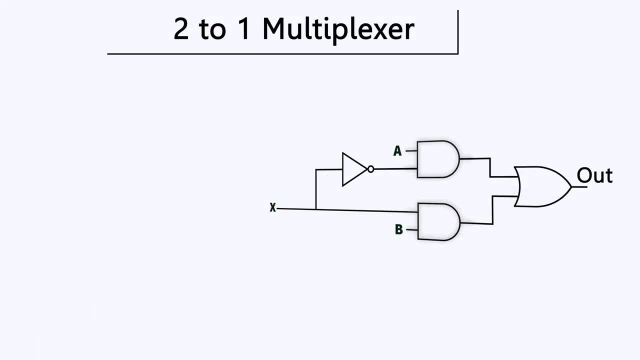 logic in Verilog versus code for combinational logic. Now, the easiest place to start with Verilog is combinational logic, So let's have a look how we can write Verilog code to describe combinational circuits. a combinational circuit which selects an output based on the value of a select pin, In this case, 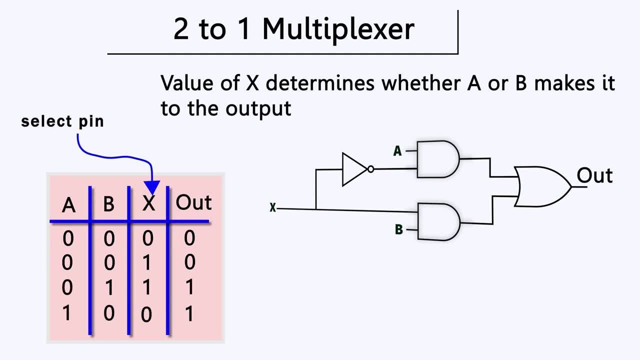 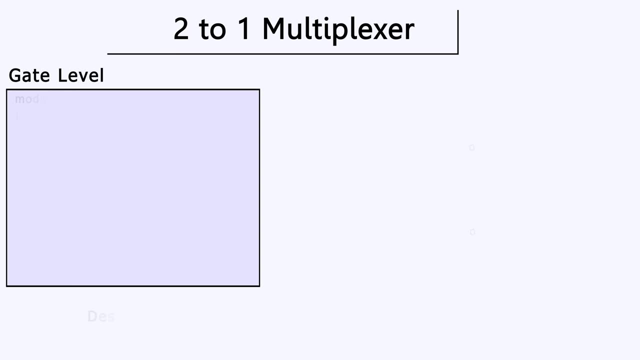 x is the select pin. if x is zero, we will select a. if x is one, we will select the output as b and as a combinational circuit, the output will change as soon as one of the inputs change. This happens almost instantaneously. So let's model this two-to-one multiplexer at the gate level and the 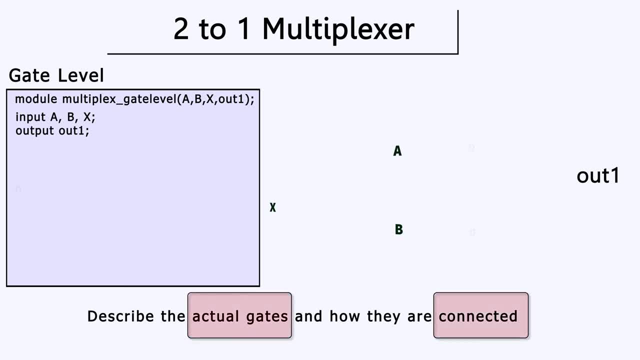 gate level we describe the actual gates and how they are connected, and modeling in Verilog at the gate level is a simple matter of instantiating each logic gate independently and then making sure they're connected together in the desired way and, as you can see, we need to create wires to make 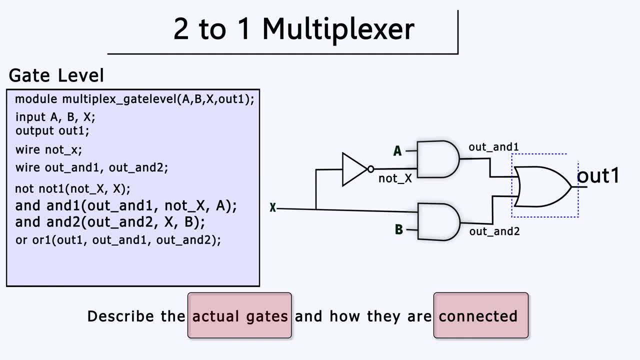 connections between gates and then just instantiate each gate. So this is a viable way of modeling circuits in Verilog but it's not very practical because sooner or later our designs are going to become much more complex. So really, gate level modeling is only good initially for very simple circuits like this, but as a starting point, knowing how to code at the 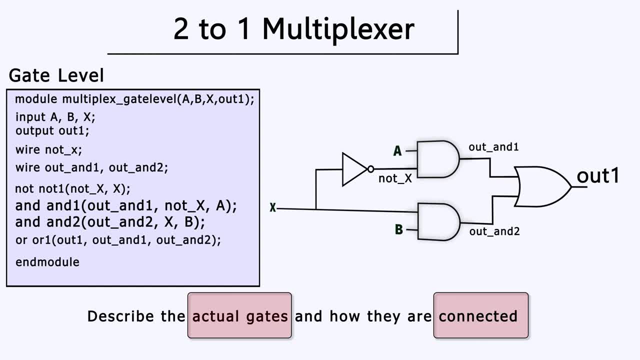 gate level is absolutely essential and we'll come back to this from time to time. And if you're new to Verilog, take a good look at the way that we define modules and the way that they're structured. Every module in Verilog looks the same and, as a hierarchical language, we piece together. 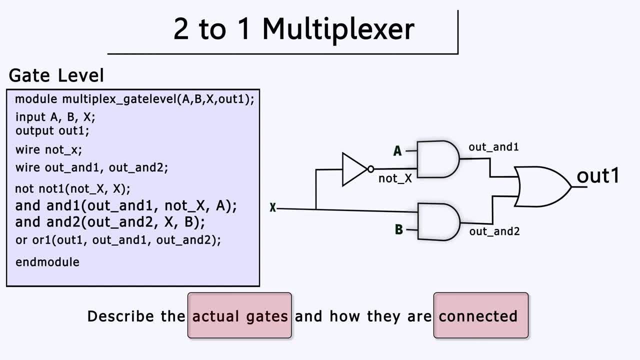 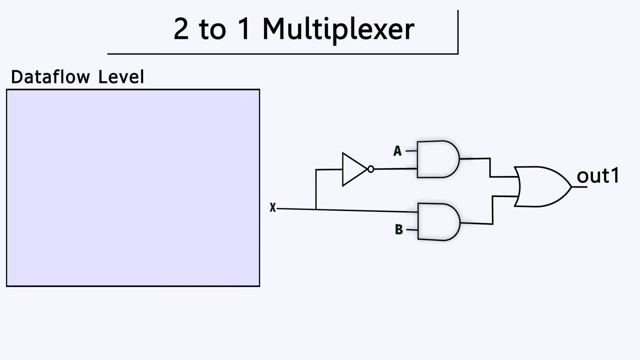 are designed by instantiating modules, So that's worth looking at at this point. Now we can also use the data flow level and this describes the flow of data in the circuit and, as you can see, we've described the two to one multiplexer using a single line of code. It's a. 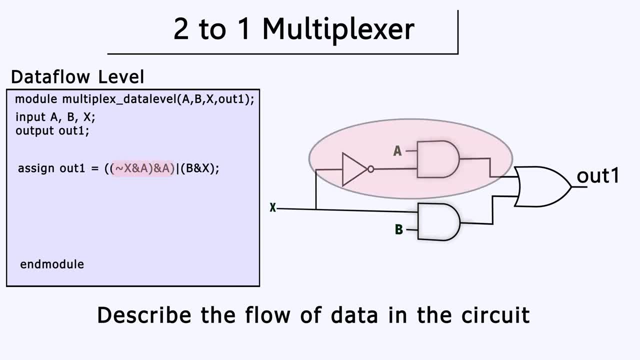 more complicated line of code, but this actually describes our two to one multiplexer. As you can see, we're using logical operators. Verilog provides a large number of these operators to almost turn our circuit into a kind of a Boolean logical sentence. So, as you can see, not X and A and A or B and X, as you can see with the 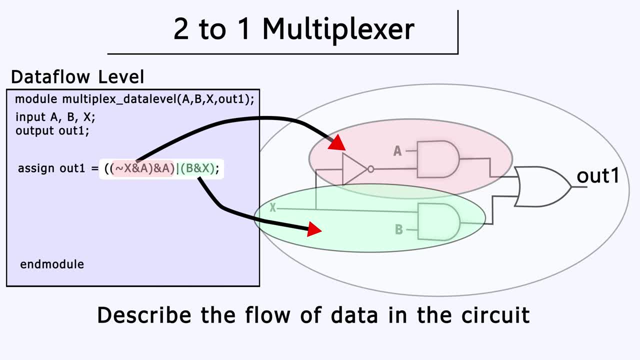 circles there. This is describing our two to one multiplexer at the data flow level. Data flow modeling is very efficient, but it can become very cryptic. What we need really is a way to describe the behavior of the circuit, rather than describing the logic gates like in the gate. 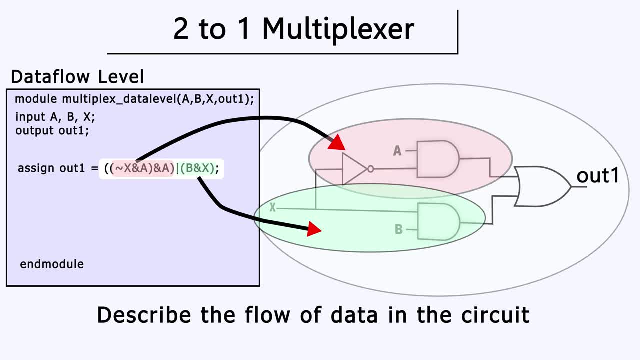 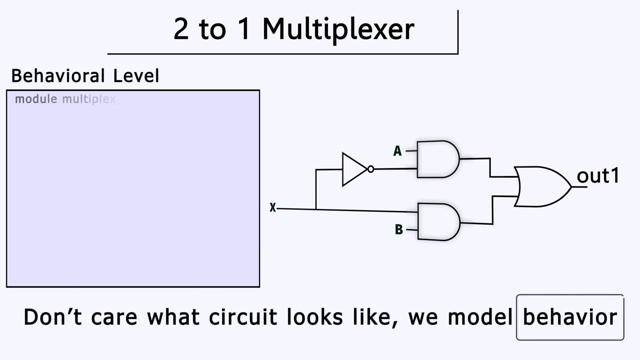 level or the flow of data in the data flow level. This is where we turn to behavioral design. The behavioral level is a much higher level of abstraction compared to the gate level and the data flow level, and here we introduce the concept of the procedural block. In this case we're using 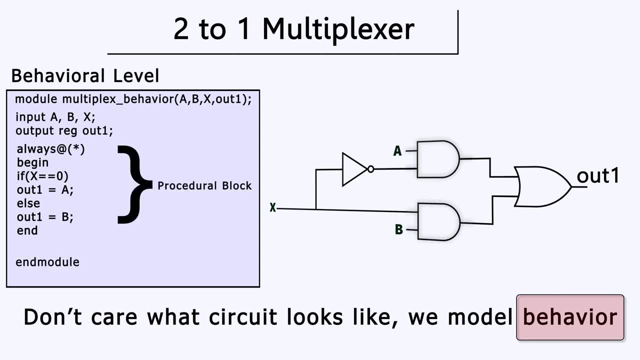 an always block, So always at, and then asterisk. That will mean the code enclosed within that always block will execute any time any of the signals change. and we can think of behavioral level Verilog code as kind of describing the behavior of the circuit rather than what the circuit actually is, And you can understand that. 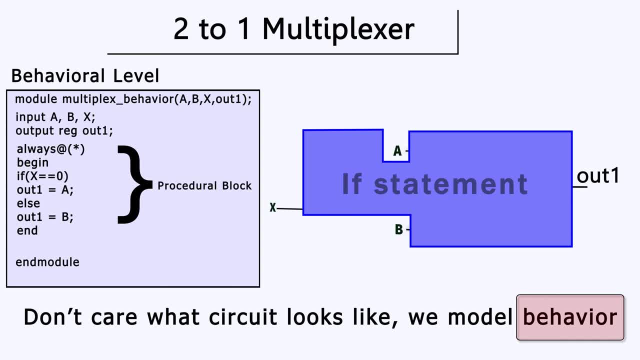 this can be a very big advantage because it's much easier to design complicated circuits when we can just describe the behavior of the circuit And we leave the complicated task of finding the actual logic gates or the the data flow level to the compiler. and as long as we trust the compiler- and I think the compiler- 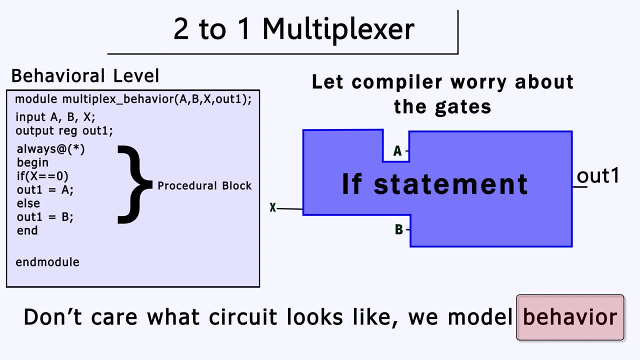 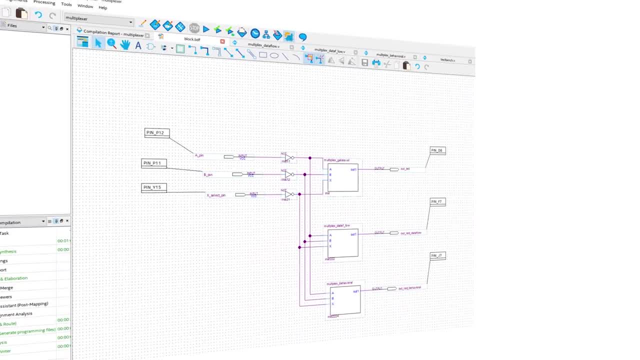 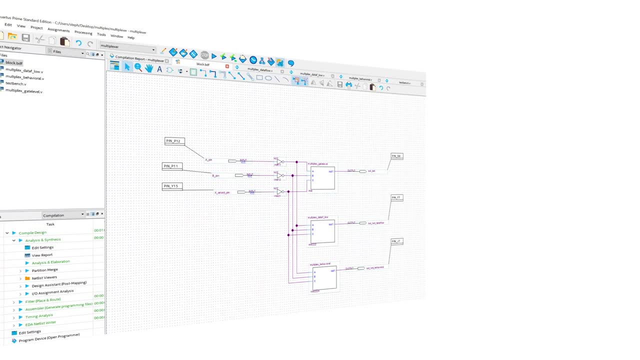 can do a much better job than I can, then working at the behavioral level is very powerful. now take a look at this. I've implemented three modules in parallel here. one of them is the gate level multiplexer, the middle one is the data flow level multiplexer and the one at the bottom is the behavioral level. 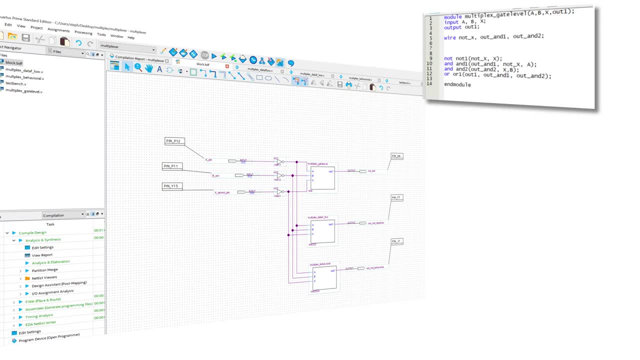 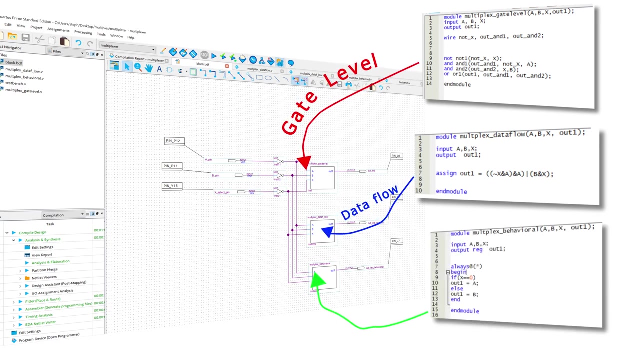 multiplexer. so it's the same module, just implemented with a different programming style. and what I'm going to do now is just check if these three modules are giving the same result, because the inputs are the same. you can see, we have three push buttons here, so a, B and X- remember, X is the select pin. those three: 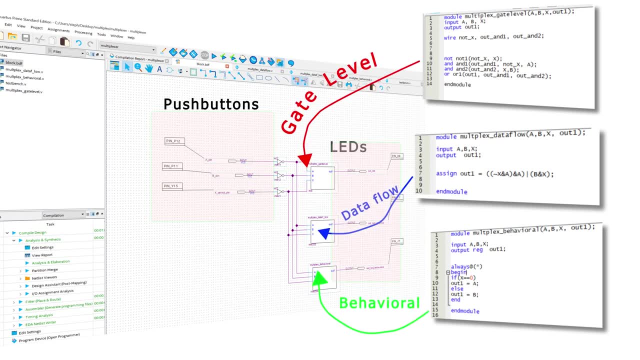 inputs are going into those three modules. you can see we have three push buttons here, so a, B and X. remember, X is the select pin. those three inputs are going into those three modules at the same time, in parallel, but the outputs are going to three different LEDs, so we're just going to verify if this is giving us the same result, for 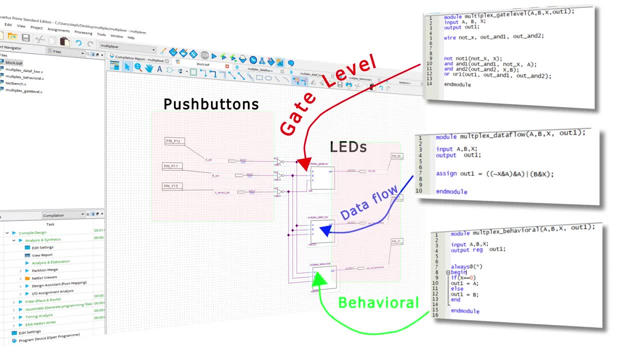 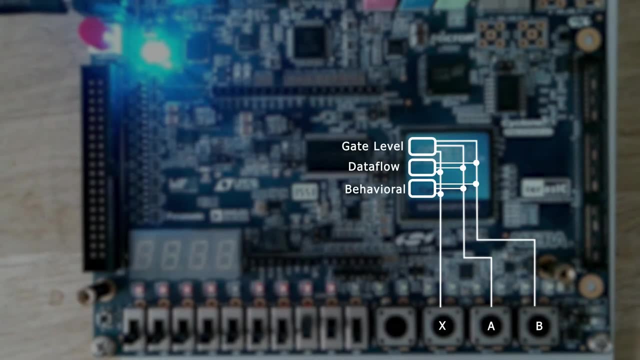 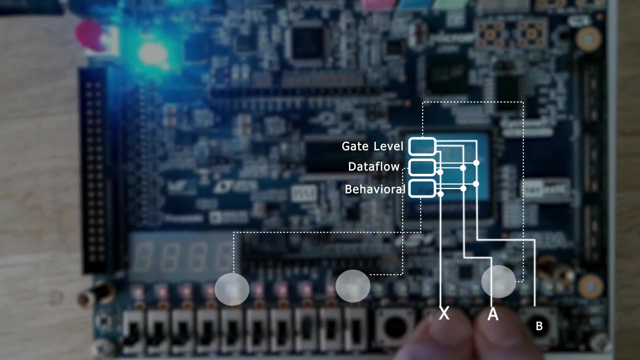 each of the three programming styles. so I've programmed this on my cyclone 5 starter kit. you can see I'm using those three push buttons for a, B and X and you can see I'm just pushing just randomly these push buttons if the LEDs light up. 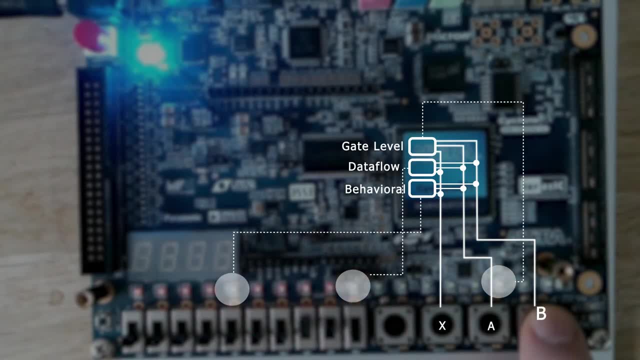 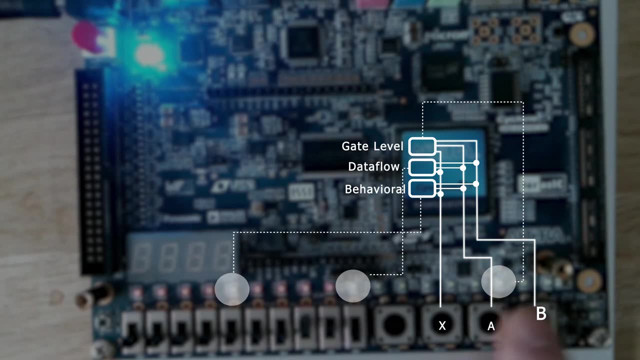 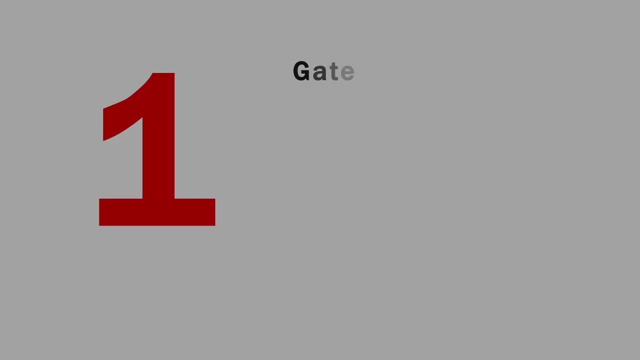 that means the output is one. now, the important thing to note here is the outputs are exactly the same. so this verifies that this multiplexer can be implemented with those three different ways: the gate level, the data flow level and the behavioral level. so let's recap: so far we've looked at combinational logic, that's logic where the output is a. 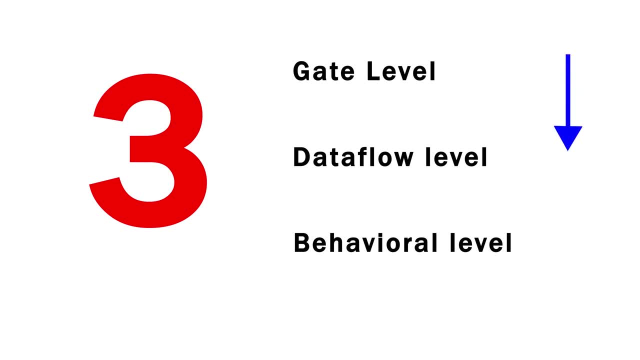 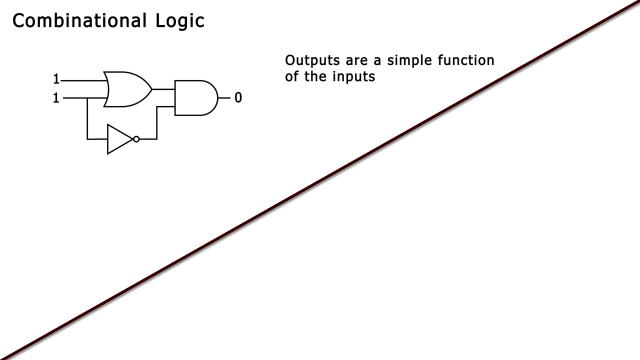 simple function of the input, and we've looked into three different ways in which we can implement combinational logic and, for an example, we use a multiplexer. there's actually another fundamental type of logic that we need to understand in Verilog and all hardware description languages. this is: 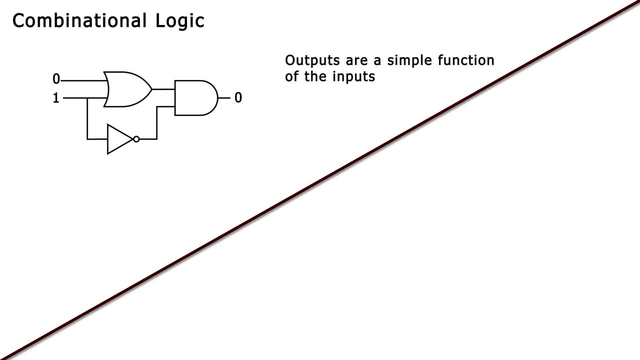 called sequential logic and, as we explained earlier on in this video, sequential logic is different because it has memory and it has a state. so the next state is a function of the current state and the inputs and if you look very closely, sequential logic is made up also of 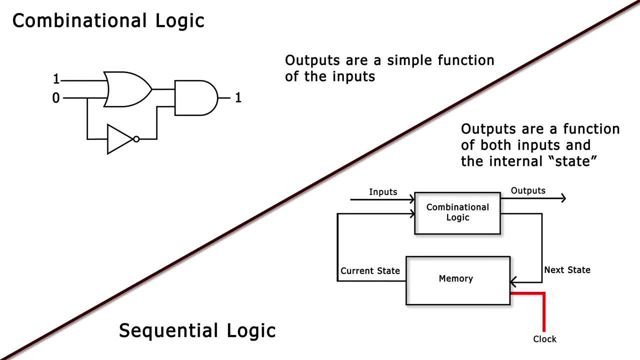 combinational logic, because that's what takes you from the current state to the next state. so, having learned how to write Verilog code for combinational logic, the question now becomes: how can we write Verilog code to realize sequential logic? well, let's start out with this very simple example. this is a 4-bit. 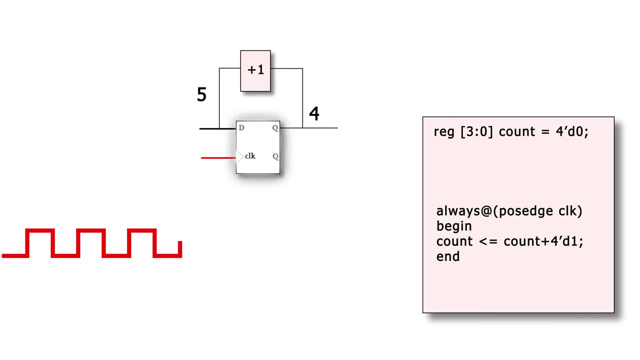 counter and you can see we're making use of a d-type flip-flop. now, d-type flip-flops are so important in sequential logic and they're basically a one clock cycle memory element, because the output Q becomes the input only on the positive edge of the clock. and you can see here: 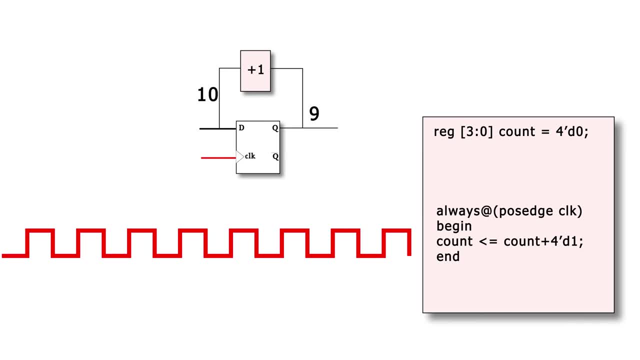 this is the memory element of our sequential logic. we also have the combinational part of our sequential logic with the plus one. this is increment in the counter. this is taking us from the current state to the next state, but you can see there's a very subtle difference between the way this 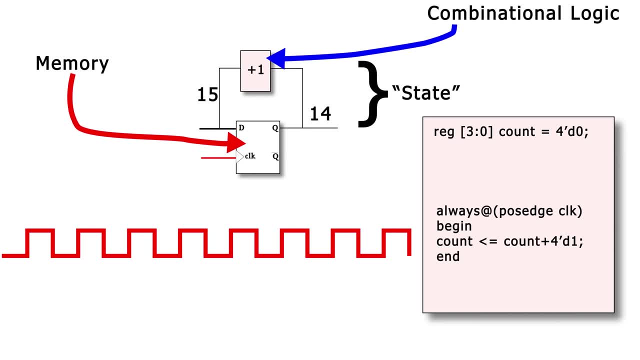 works and the way combinational logic alone works. so we're going to start out with the d-type flip-flops, and it's all based on the concept of a state and the necessity of this one clock cycle memory element called the d-type flip-flop. now, 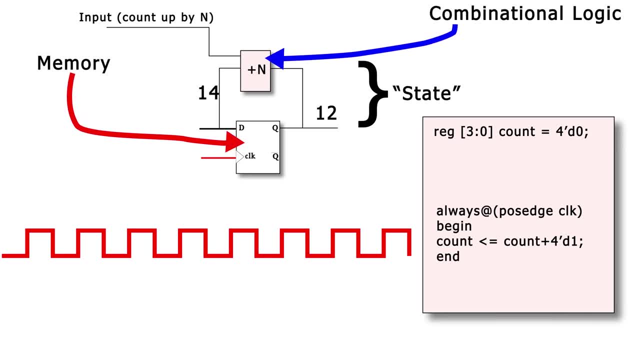 take a look at the code. we're using a procedural block, but this time the sensitivity list has positive edge of clock, which means the code within that block will only execute on the positive edge of the clock. but have a look at this symbol that we're using. this is called the non-blocking assignment and 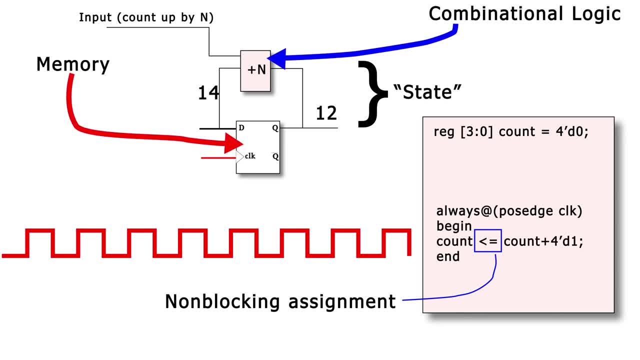 this is different to the assignments we've been using, previously called the blocking assignments, and if you use this assignment, this will be synthesized in hardware as sequential logic and the key to it really is this non-blocking assignment. so let's take a closer look at what exactly a 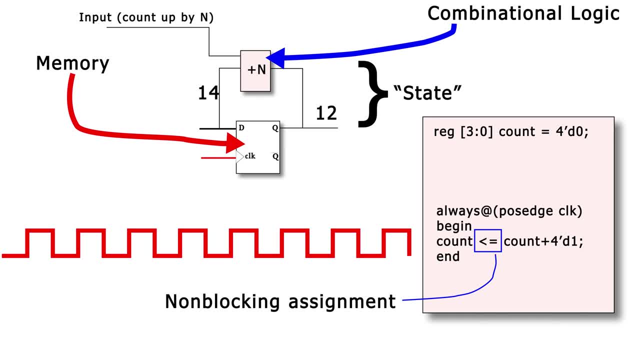 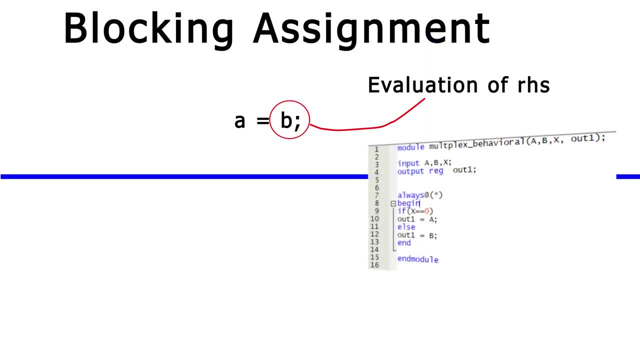 non-blocking assignment is and how it works and, importantly, how is it different to a blocking assignment? now, the blocking assignment, you have a valuation of the right-hand side and then assignment to the left-hand side, and this is exactly what we want with combinational logic, but with the 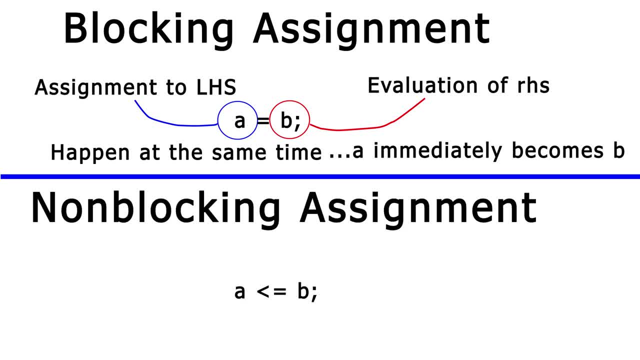 non-blocking assignment. we have separation between the evaluation of the right-hand side, which is immediate, and then assignment of the left-hand side. the assignment to the left-hand side is delayed until all other evaluations of the right-hand side are completed in that particular time step. so let's take 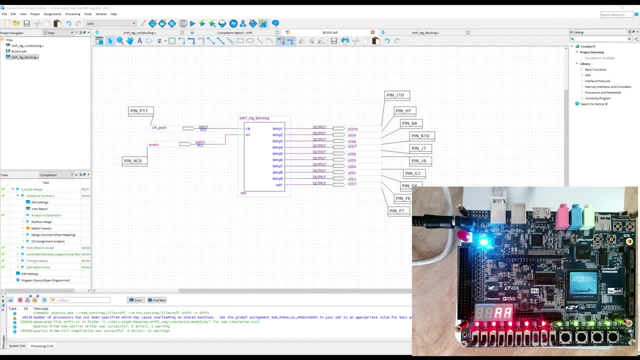 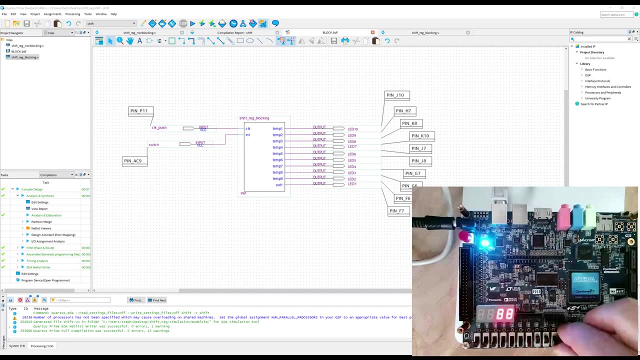 a look at this design in a more specific way in the next slide, which is this one. Now, what I've got here is a push button clock which will give a positive edge every time the push button is pushed and released, And I also have one of these side switches, and these will either be one or zero, depending on which position they're in. 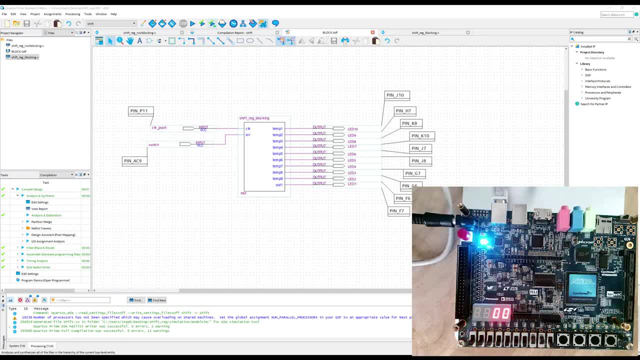 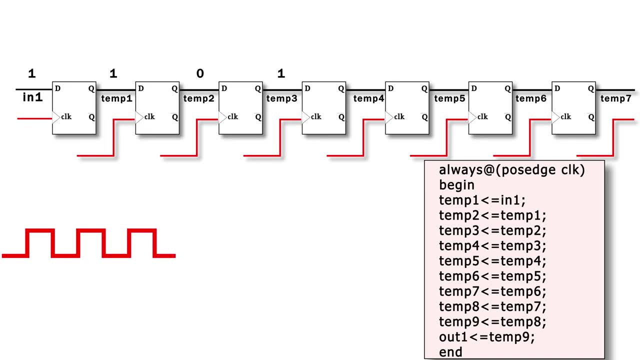 And what I'm sort of modeling here is a shift register And I've got a version of this shift register which is using non-blocking assignments And, of course, what will happen, hopefully, is the bits will cascade through the shift register, one D-type flip-flop at a time. 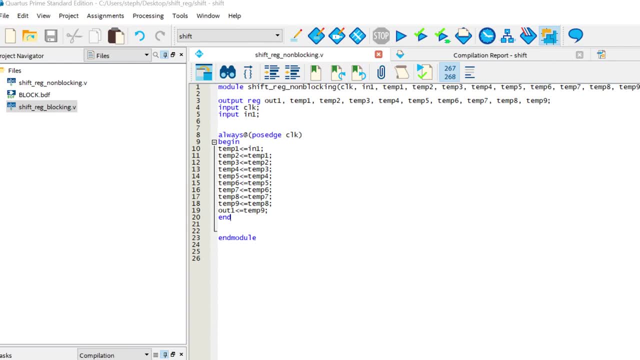 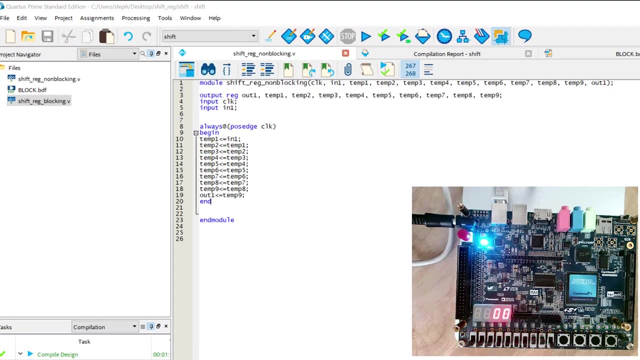 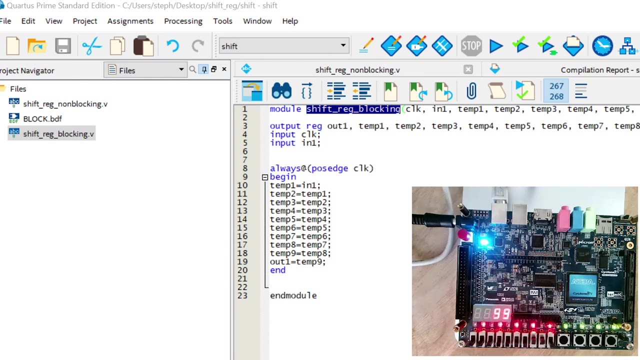 But it will only happen on the positive edge of the clock. Now I've also got another version of this design, but this time we're using blocking assignments instead of non-blocking assignments, So we're going to investigate the difference in the way that the compiler synthesizes these two designs. 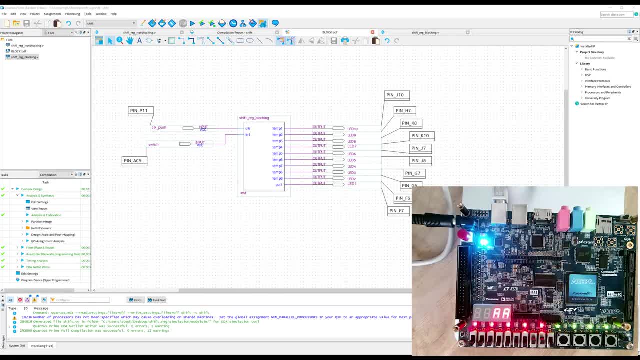 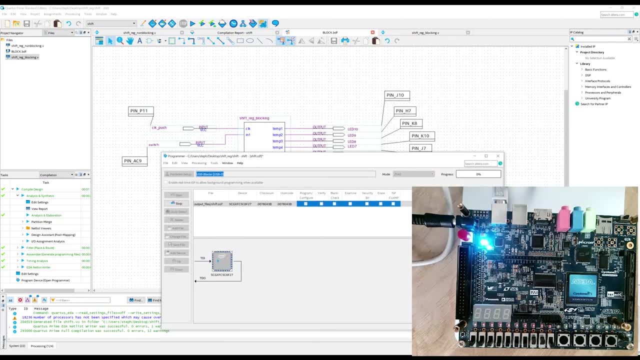 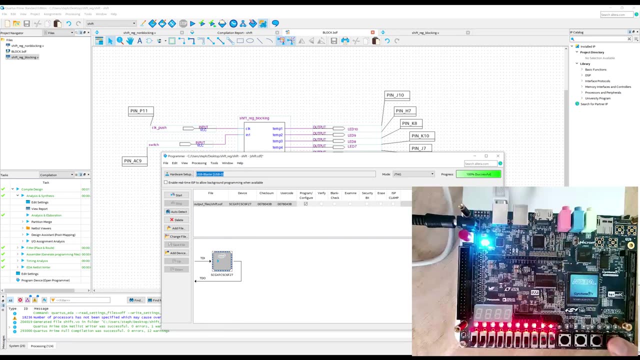 So let's take a look. So I'm going to open up the programmer. Let's program the device Now. the first one I'm looking at is the blocking assignment. So the push button clock is this one. If I move the side switch there you can see all of those LEDs light up. 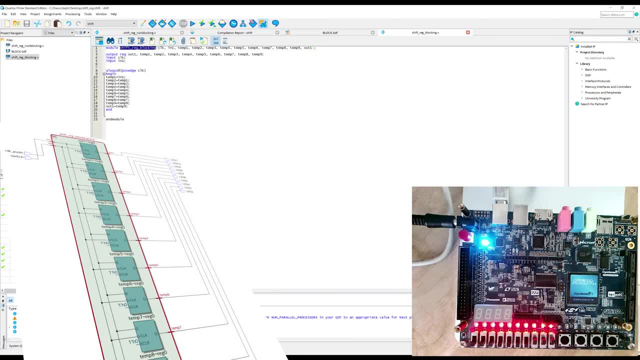 And that means, if there's one going into this design, everything becomes one instantly. OK. and really, what's going on is these? Well, the way the computer works, The way the compiler is synthesizing, this is as parallel D-type flip-flops. 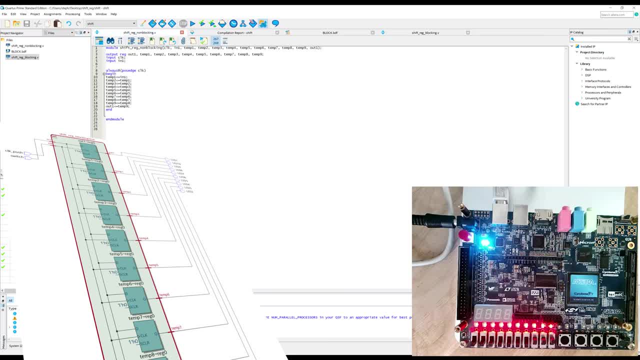 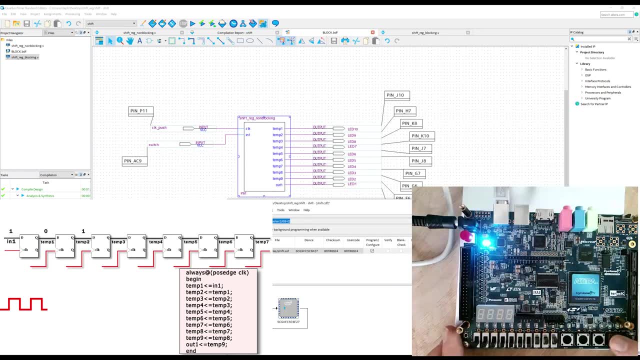 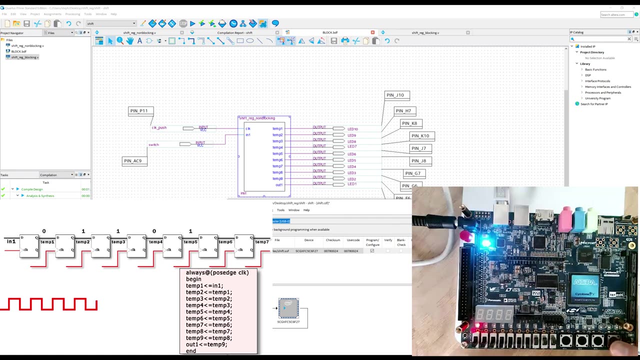 Now let's have a look at the other version of this design, this time with non-blocking assignments. So this is the non-blocking assignment case. If I press the clock, we get one bit going into the shift register, But, unlike the blocking case, we don't get all the LEDs lighting up straight away. 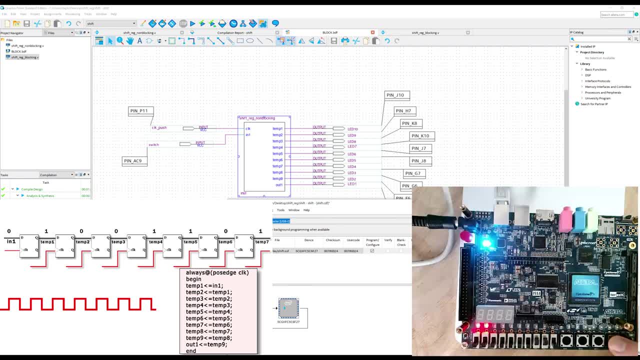 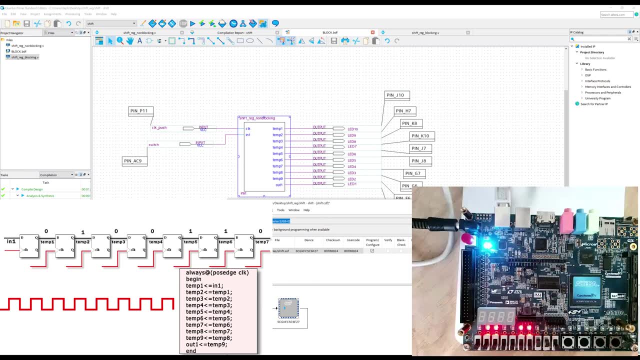 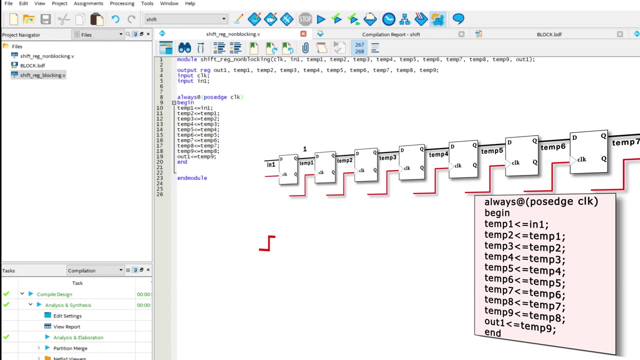 If I click the clock I make the input zero. Now you can see it's shifting one clock cycle at a time and filling up in a sequential manner. So this is the fundamental difference between the blocking assignment and the non-blocking assignment And, as I said before, the reason we get the desired behavior from the non-blocking assignment shift register is because we have separate blocks. 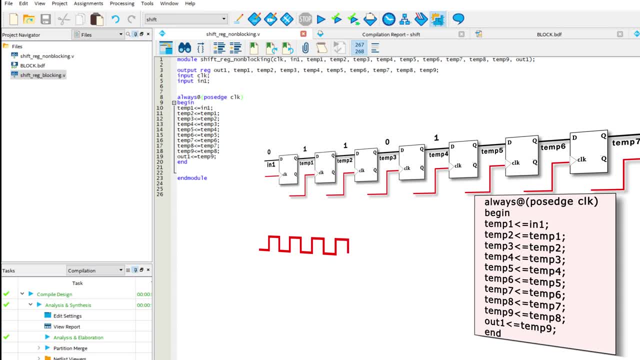 Because we have separation between the evaluation of all the right-hand sides and the assignment. Now have a look at this shift register. All of the right-hand sides are evaluated And what that means in hardware is they get loaded into the D-type flip-flop. 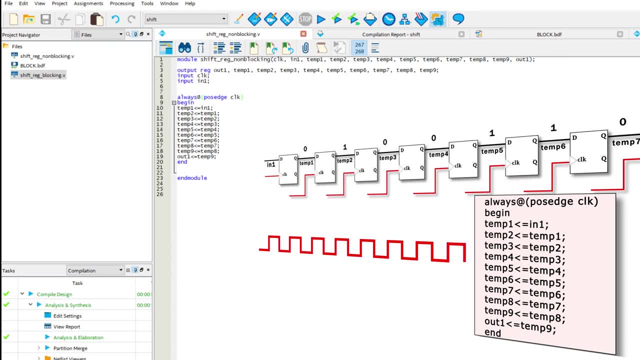 The assignment to the left-hand side, which in practice means the bits shifting to the right, That only takes place on the positive edge of the clock, But when we try to use blocking assignments to do this, the evaluation of the right-hand side and the assignment to the left-hand side. 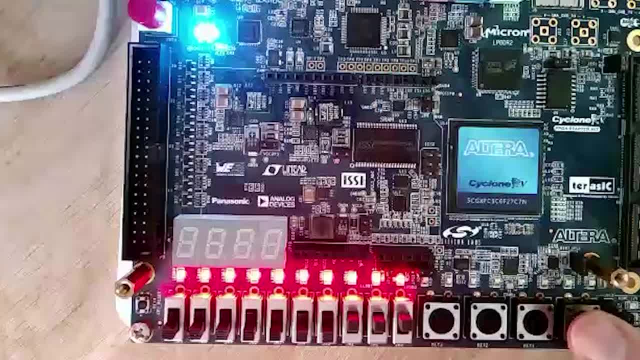 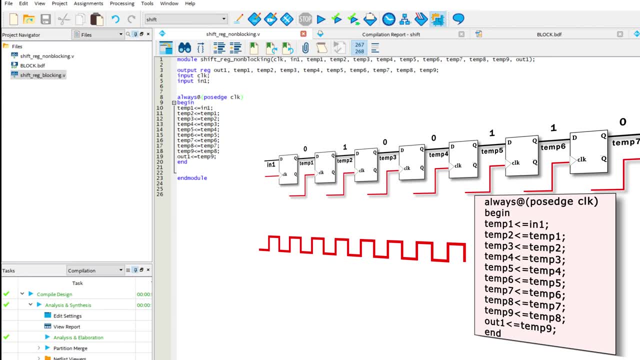 Happened immediately, And that means all of our LEDs lit up. We did not get this one clock cycle: cascade through the shift register. Okay, And this is because we have the immediate assignment to the left-hand side. And then you move on to the next statement. 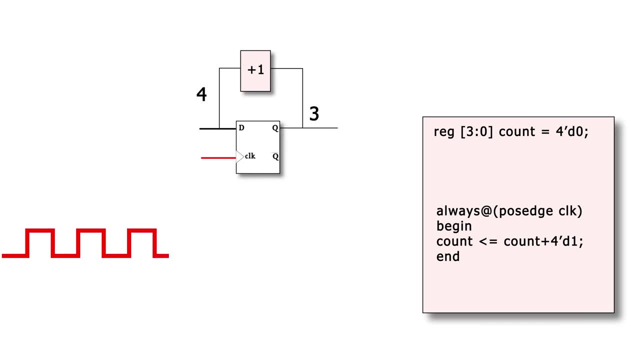 Okay, And that's not what we want in sequential logic, But in combinational logic, that's exactly what we want. For example, we know that the output should change instantaneously And that propagation of information Through the gates is instantaneous. 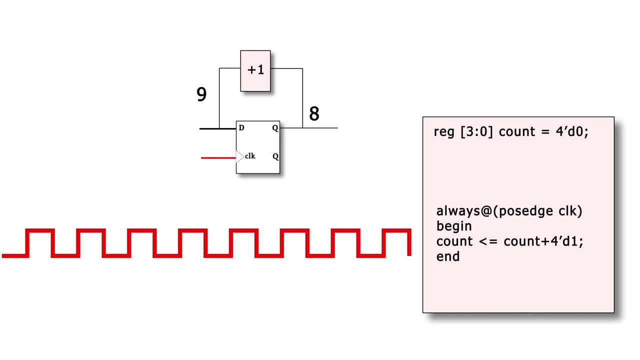 But in sequential logic we always have to keep in mind that we need a non-blocking assignment Because we need that Well, at least one clock cycle memory element to coordinate the movement from the current state to the next state. And this is why the general rule for procedural assignments in behavioral modeling is when you want combinational logic. 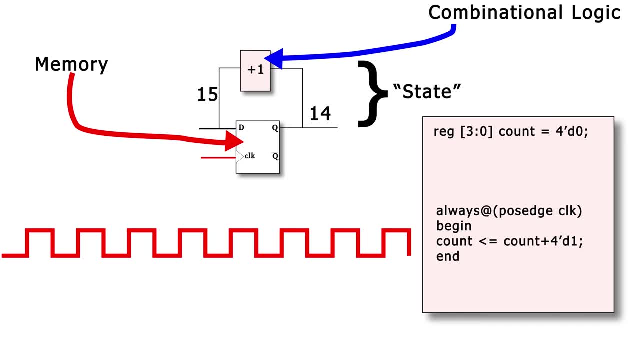 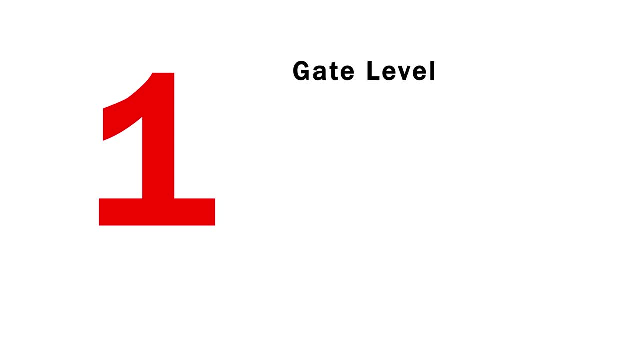 You should use blocking assignments, And when you want sequential logic, You should use non-blocking assignments. So just to recap, We've talked about the three different ways that you can write code in Verilog: The gate level, The data flow level. 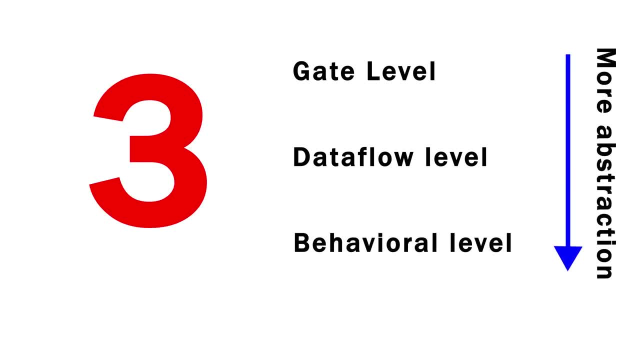 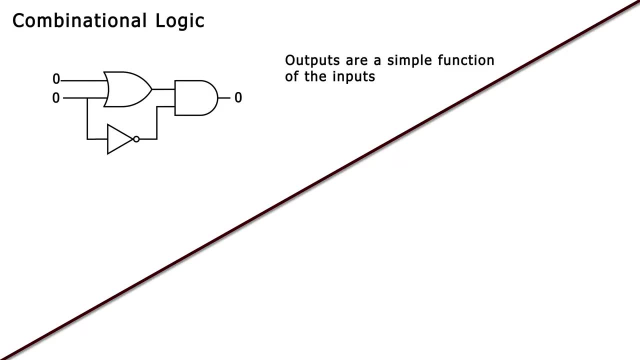 And the behavioral level. Then we introduced the idea of the procedural block And we said that we need to be careful about the way that we use blocking assignments and non-blocking assignments, Because blocking assignments give us combinational logic And non-blocking assignments give us sequential logic. 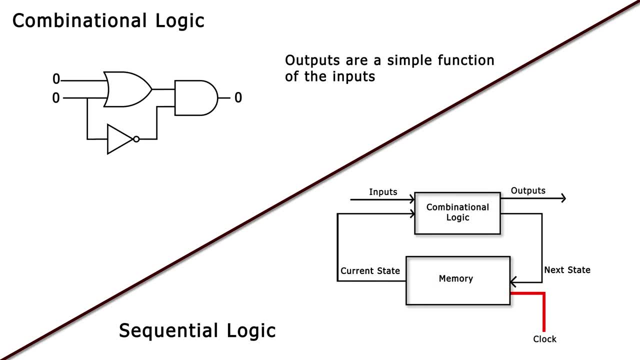 So you have to know what you're doing. We also talked about the fundamental difference between combinational and sequential logic, But I think that's all I wanted to talk about in this video, And I think we've gone through some of the most important concepts in Verilog coding. 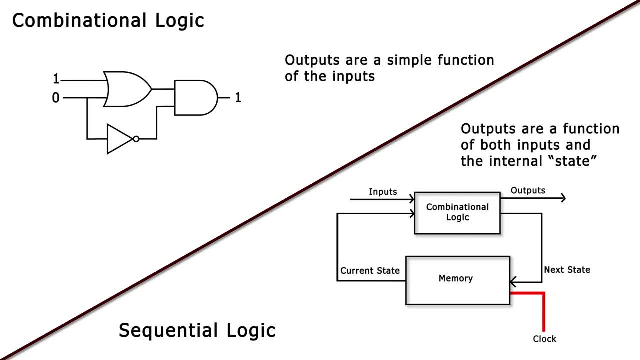 And I hope this was useful to you. Thank you for watching And I'll see you next time. Thank you for watching.